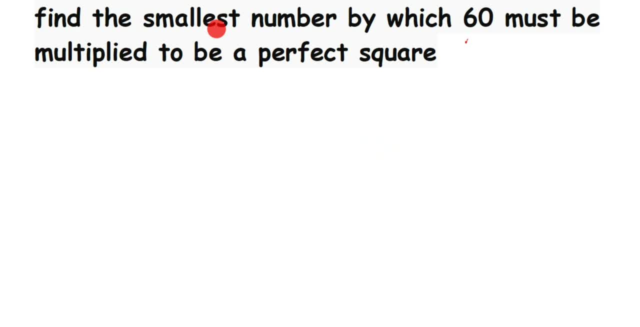 have to solve this. So in case they ask you what is the smallest number to be multiplied or divide, then you have to use prime factorization method right Now. in case they ask you find the smallest number to be added and subtracted, In that case you have to use a division method. 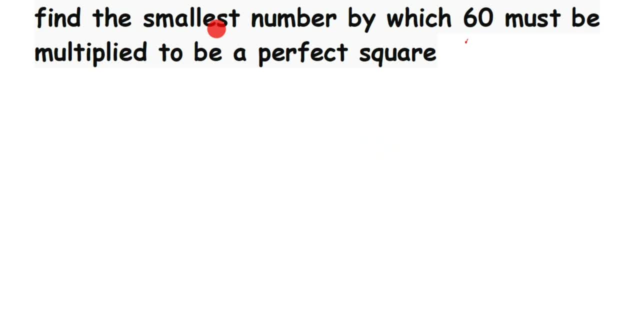 So here I am going to use a prime factorization method, because they are asking smallest number to be multiplied. So we are going to find the prime factorization of 60.. So here we go. So 60 is a small number. Now we are going to do a prime factorization, So we 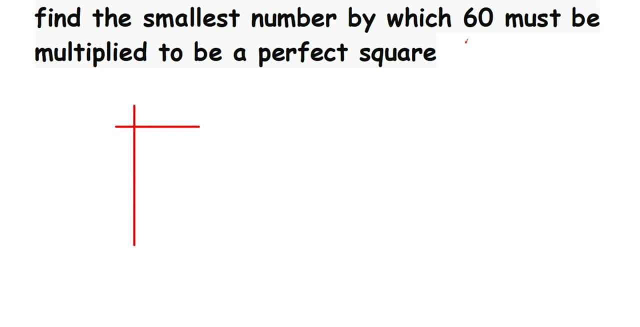 should take only prime numbers. So here we have 60. I am going to start with 2, because it goes in 2 tables. So 2 is a prime factorization. So here we have 60. I am going to start with. 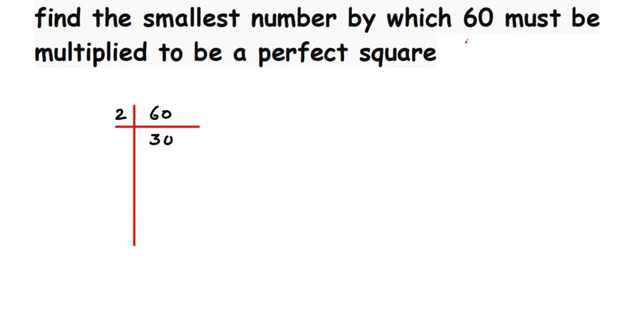 3s are 6, then write down the 0. we got 30. so again 30 goes in 2 table. 2 15s are 30. again 15 doesn't go in 2 table. so next prime number is 3, so 3 5s are 15 and then 5 doesn't. 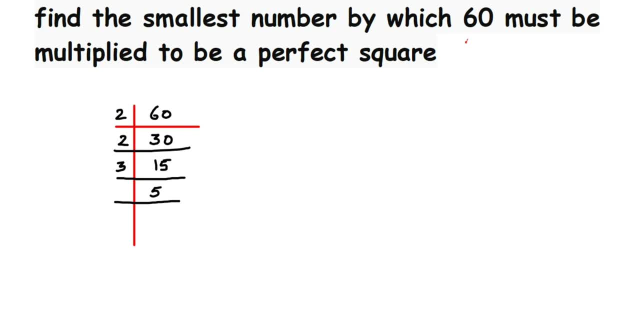 go in any other table except itself. so 5 1s are 5 now, 60 is equal to what i got here, 60 is equal to 2 into 2, into 3, into 5. right now, if you see the perfect square numbers, the prime factors, what you. 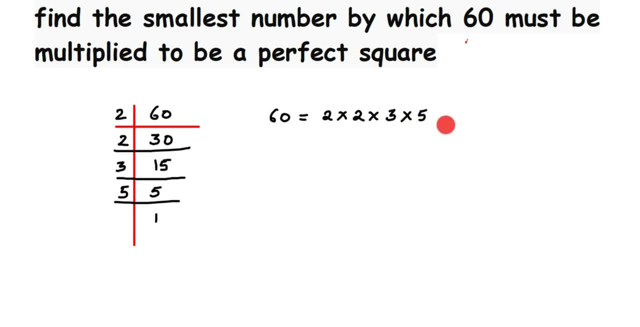 got here, they will be in a proper pair. okay, proper pair means, for example, let me take 16 here. okay, i'm just taking example 16, so 16 will be equal to 2 into 2, into 2 into 2. yeah, so you can see, i got. 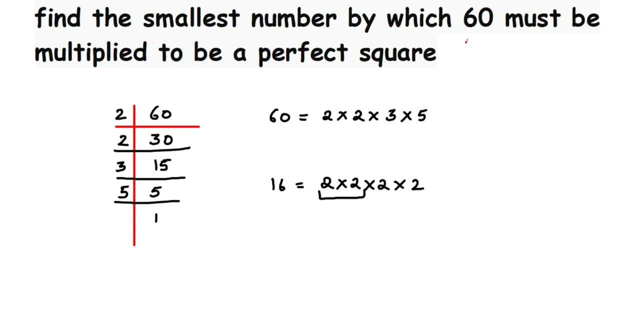 a pair. of this is first pair and this is second pair, right. so here, if you see, 60 is not perfect square. i'm not getting the factors in pair. i got one pair of two. pair means in a set you should have a same common factor, the same factors, right? so two for. 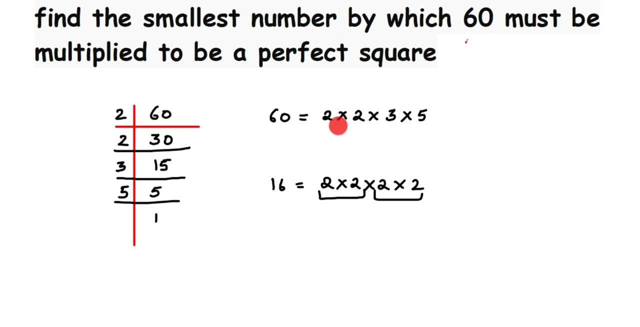 two. i got one set, but for three and five there is a no pairing right. so to get to make it perfect square, i want one more three and i want one more five. so perfect square numbers are gonna have a proper pair of prime factors. but here it is not there, so i have to introduce one more three. 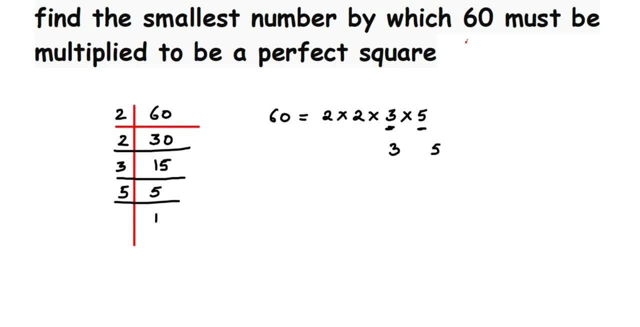 and one more five, so that there will be a proper pairing and the number will become perfect square. so i have to multiply here with one more three and one more five. got it. so same three and five are going to multiply on the left side also, because you cannot do everything on right side. 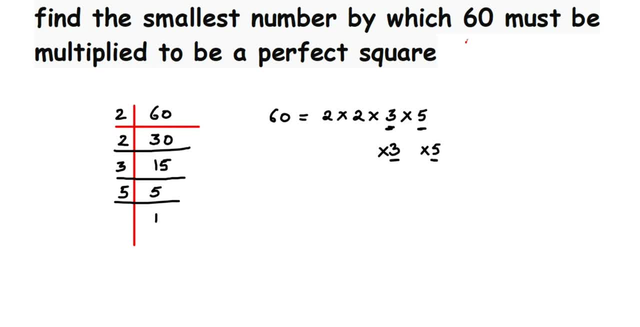 it should be balanced. whatever you're doing on the right side, you should do on the left side also. so let me just erase this. so here 60 is equal to like two into two. let me just write down, then three into and then into five into. okay, so here i have to multiply with one, three and i have 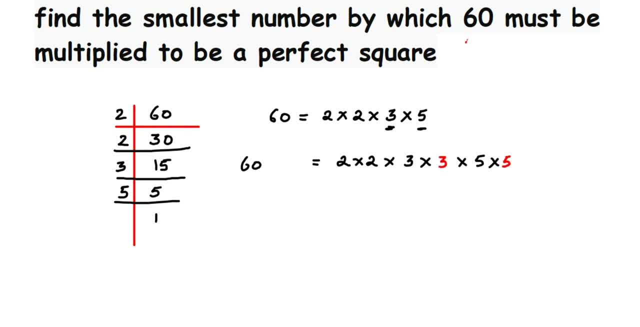 to multiply here with one five, so that you can see this is forming a one pair. this is forming a one pair and this is forming a pair. i got a proper pair right, and so i have introduced three and five here. same three and five. i'm going to multiply on the left side also. that's it now. 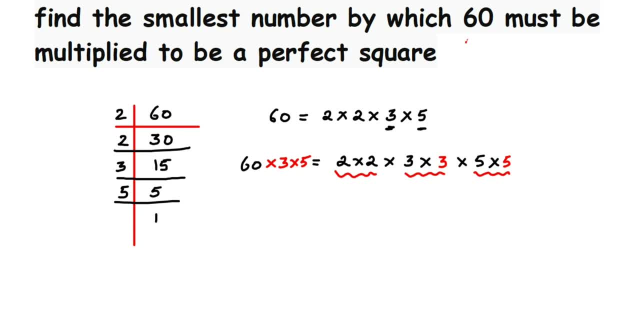 they have asked you what is the smallest number to be multiplied. so i have multiplied two numbers: one is three and one is five. so three fives are 15.. so 15 is the smallest number by which you should multiply with 60 to get perfect square. i hope it's clear. now we're going to multiply this. 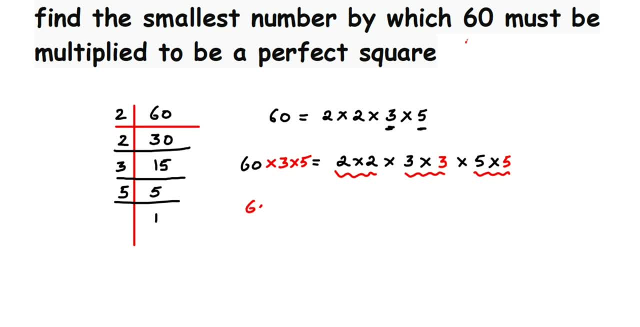 so here we'll get: 60 multiplied by 15 is equal to. so 2 into 2, into 3, into 3, into 5, into 5. now, 60 into 15 will be 900, 15, 6 is 90, so 90, and then 1, 0 so 900, so 900 is equal to the same thing. 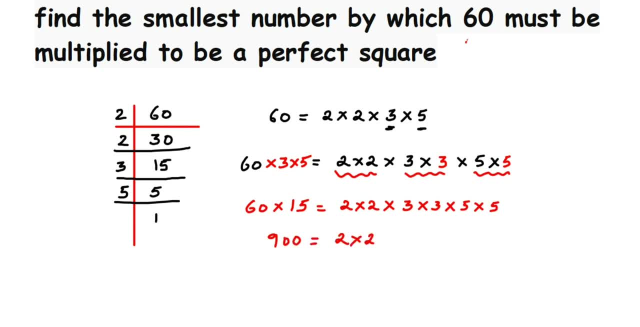 2 into 2. now you can see we are getting a proper pair here: 3 and then here i got 5 into 5. now this is not necessary. your answer will end up here. what is the smallest number to be multiplied? it is 15.. i hope it's clear. we have multiplied 3, 5 as 15.. it's not 3, it is not 5, since we have got two.